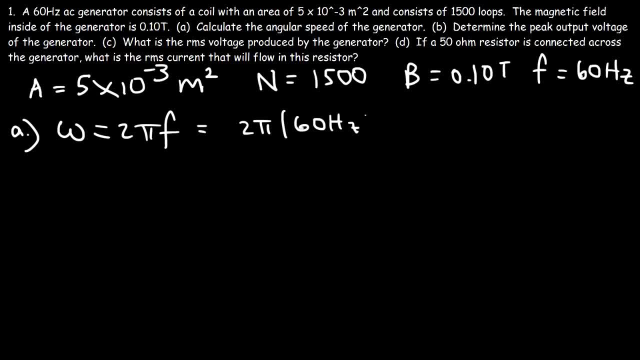 it's 2 pi times the frequency, which is 60 Hertz, And so that's going to be about 377 radians per second, And so that's all you need to do for the first part of the problem. Now let's move on to the next. 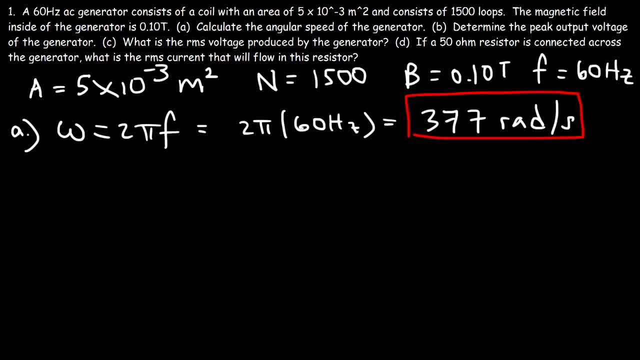 part, Determine the peak output voltage of the generator. So the formula that we need is this equation: The peak output voltage is going to be NBA times Omega. Now for an AC generator, we have a sinusoidal function, and so it alternates like this: And so here is the peak voltage. Now this graph can be: 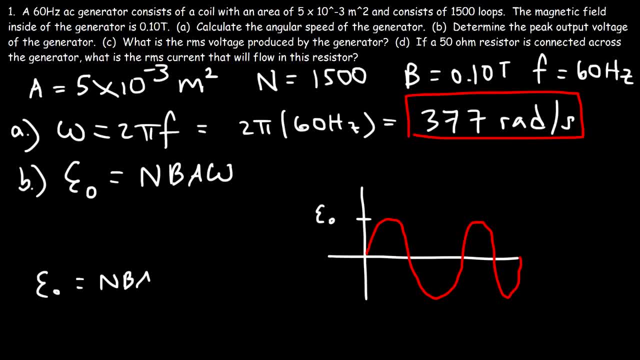 described by this formula. It's NBA times, Omega times. sine of omega t. because it's a sinusoidal function, It varies with time. However, if we wish to calculate just a maximum EMF, we just need to use this formula. We don't need the sine portion of it. Sine 90 is 1, so at its maximum value we can. 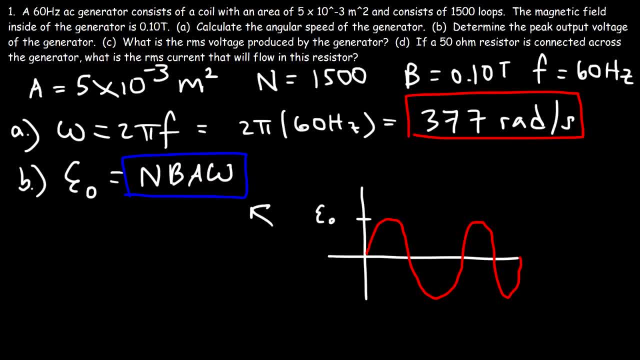 replace sine with 1.. And so that gives us this equation. Now a DC generator is going to have an output that looks like this, So it's only on the top portion of the graph, And this is for an AC generator. So in this problem, n is 1500, b is 0.10, the area is 5 times 10 to the minus 3, or 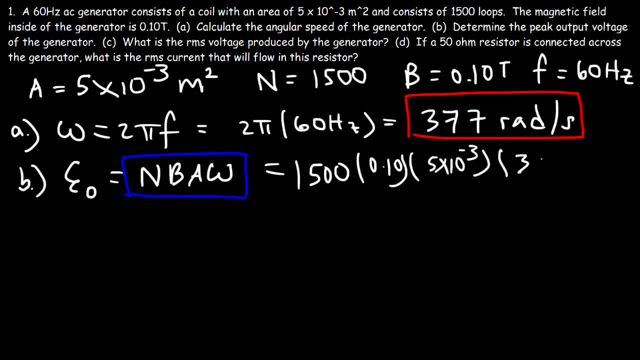 0.005, and the angular speed is 377.. Ratings per second. So let's multiply these four numbers together, and so you should get 282.75 volts. So that's the peak output of this particular AC generator. Now, what about Part C? What is the RMS voltage? 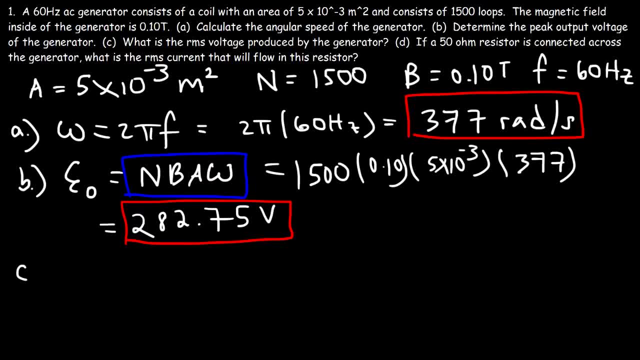 What is the RMS voltage produced by the generator? The RMS voltage is equal to the peak voltage divided by the square root of 2.. So it's 282.75 divided by the square root of 2, and that comes out to be 199.9 volts. And so that's it for Part C. 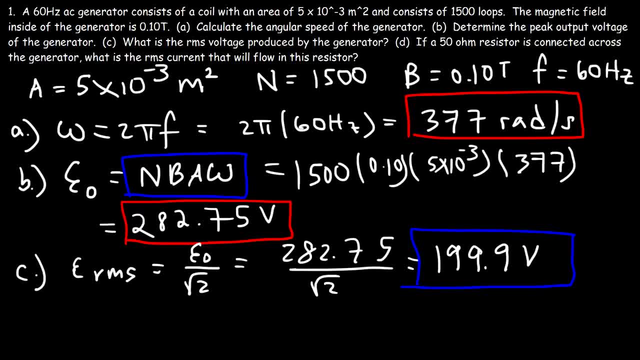 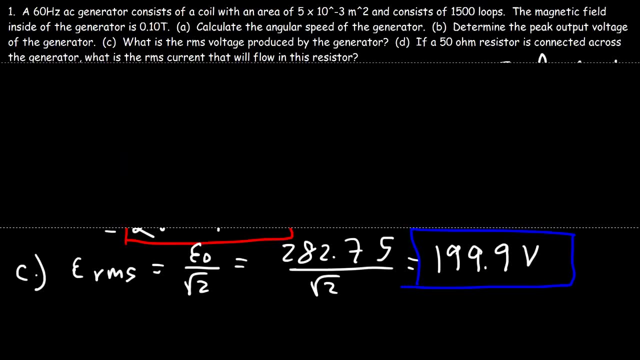 Now let's move on to Part D. If a 50-ohm resistor is connected across the generator, what is the RMS current that will flow in this resistor? So let's draw a picture first. So let's say if we have a sine wave. 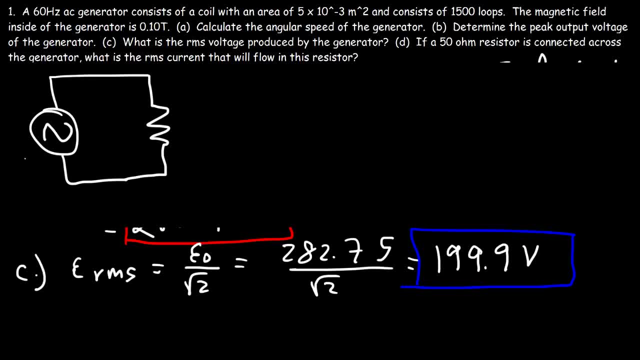 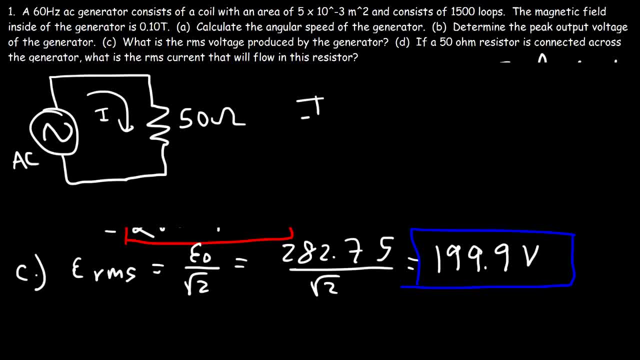 So to calculate the current, we know we could use this equation: V is equal to IR, So the current is going to be the voltage divided by the resistance. So we're going to use the RMS voltage generated by the generator and divided by the resistance. 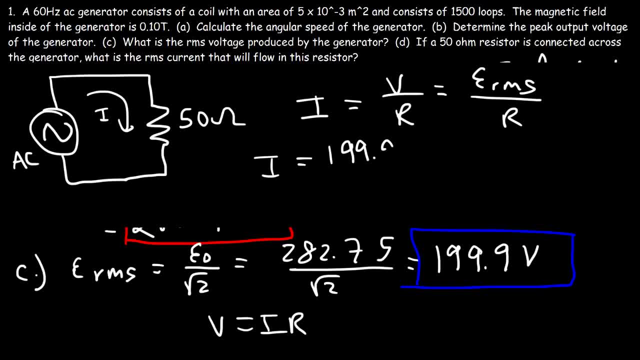 across it. So it's 199.9 volts divided by 50 ohms. Now, because we use the RMS voltage, this will give us the RMS current in the circuit. So this is 3.998, which we can round and say it's 4 amps. 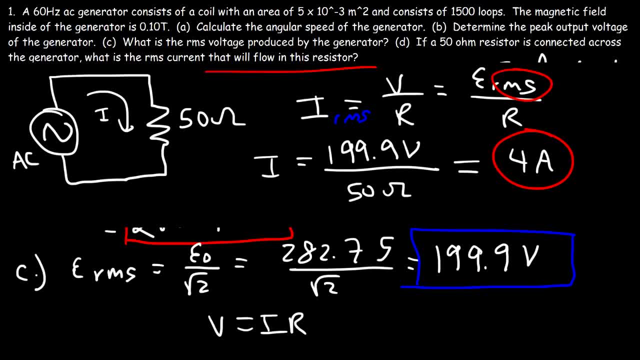 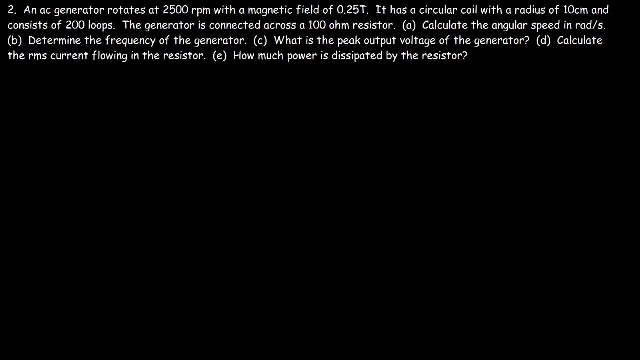 So that's the current that's going to flow in this particular resistor, Number two, an AC generator rotates at 2500 RPM with a magnetic field of 0.25 Tesla. It has a circular coil with a radius of 10 centimeters. 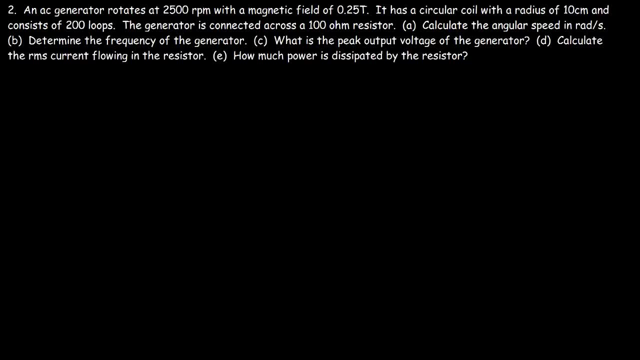 And consists of 200 loops. The generator is connected across a 100 ohm resistor. Calculate the angular speed in radians per second. So let's start with that first. So right now the angular speed is in RPMs, rotations per minute, or you can use revolutions per minute. 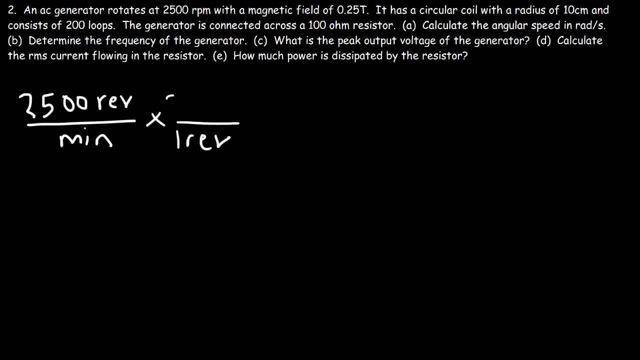 Now one revolution is 2 pi radians, So we can cancel these units. And one minute is equal to 60 seconds, And so this is how you can convert RPMs to radians per second. You need to multiply it by 2 pi and then divide it by 60.. 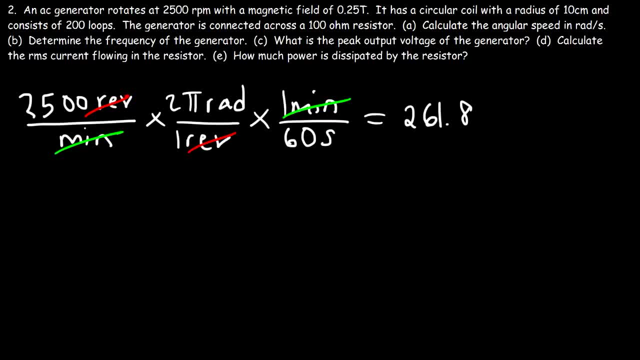 And so the angular speed is 261.8 radians per second. And so that's the answer for problem number two, And that's the answer for part A. Part B determine the frequency of the generator. So we know that the angular frequency is equal to 2 pi f. 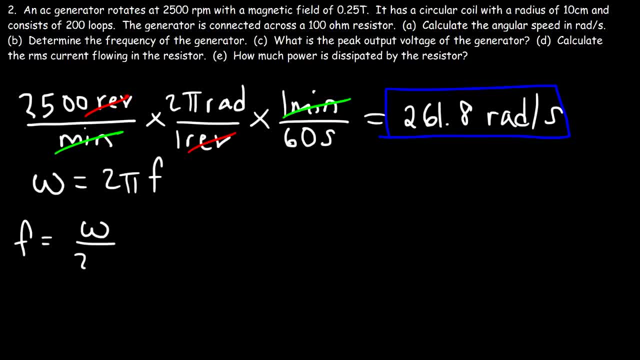 So to calculate the frequency, it's omega divided by 2 pi, So it's going to be 261.8 radians per second divided by 2 pi, And so that's going to be 41.67 hertz. So now you know how to convert from RPM to frequency for a generator. 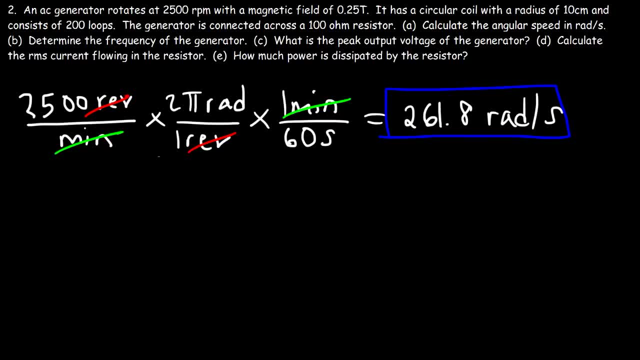 Now let's move on to part C. What is the peak output voltage of the generator? So we could use this equation: It's equal to nba times omega. So in this example there are 200 loops. The strength of the magnetic field is 0.25 tesla. 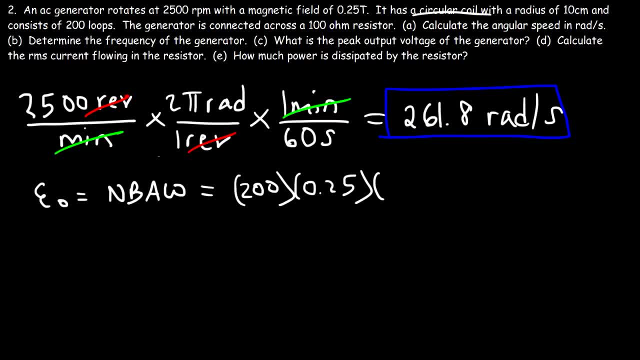 And the area. we have a circular coil, So the area is pi? r squared. The radius is 10 centimeters. We need to divide that by 100. And so that's going to be 0.10 meters. And don't forget to square it. 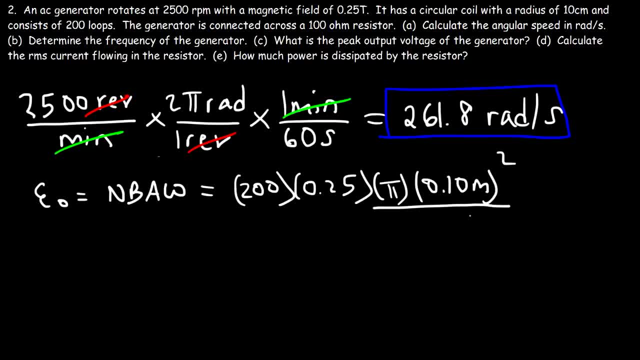 So this represents the area of the circular coil Times omega which we have. That's 261.8.. So the peak output voltage is 411.2 volts. So that's it for part C. D. Calculate the RMS current flowing in the resistor. 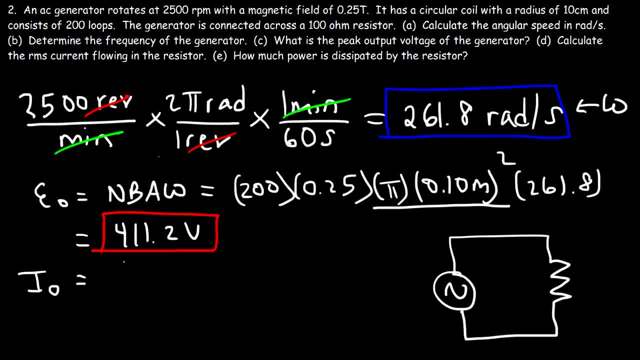 So first let's calculate the peak current. It's going to be The peak output voltage divided by the resistance. So keep in mind V is equal to IR. If you want to calculate the current, it's the voltage divided by the resistance. 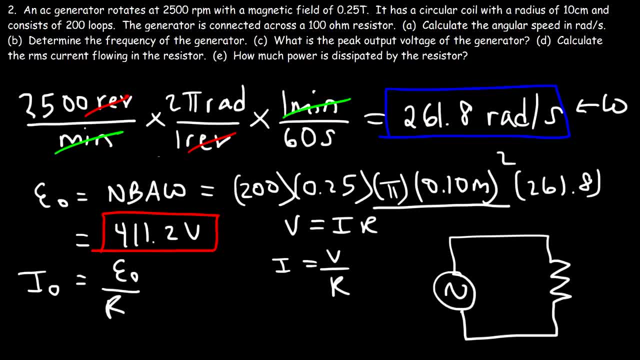 And this represents the voltage produced by the generator. So the voltage of the generator is 411.2. And the resistance is 100 ohms. So this is going to be 4.112 amps. So that's the peak current. Now to calculate the RMS current. 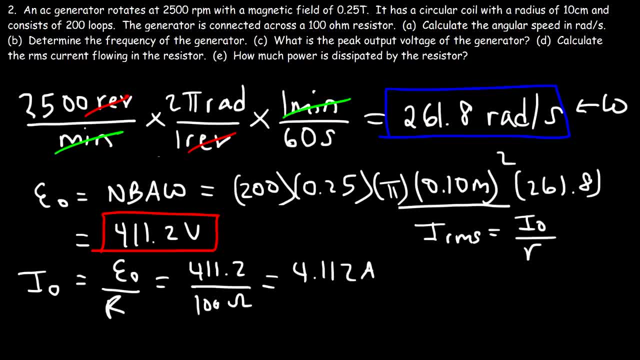 it's going to be the peak current divided by the square root of 2.. So that's 4.112 amps divided by the square root of 2.. And so that's going to be 2.908 amps. So that's it for part D. 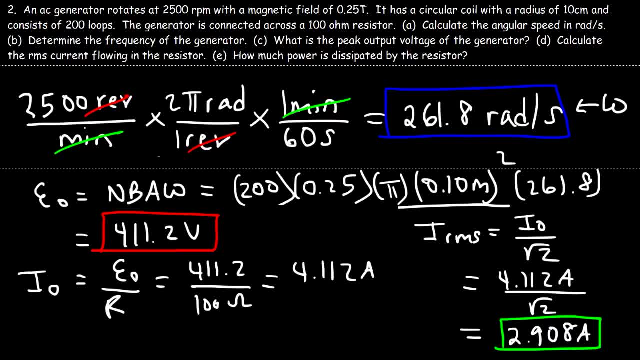 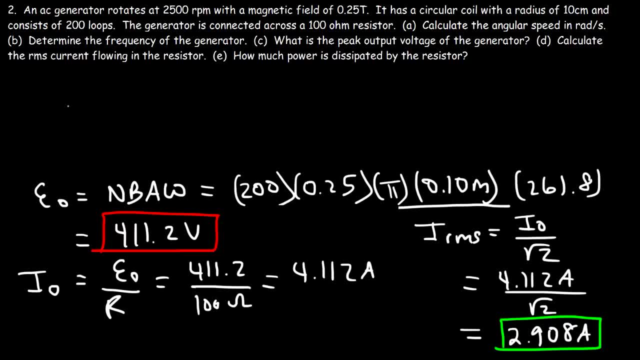 Now let's move on to part E. How much power is dissipated by the resistor? So we can use this formula: It's I squared times R, So we need to use the RMS current. If you use the peak current it would be 1 half I squared R. 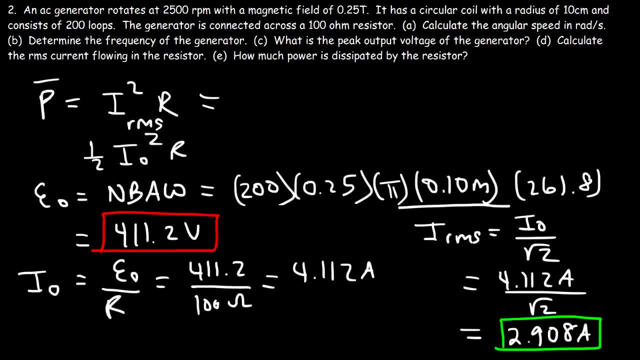 And this will give us the average power. So The RMS current is 2.908 squared times 100.. And so the average power dissipated by the resistor is 845.6 watts. If we use the other formula, 1 half of the peak current, 4.112 squared times 100.. 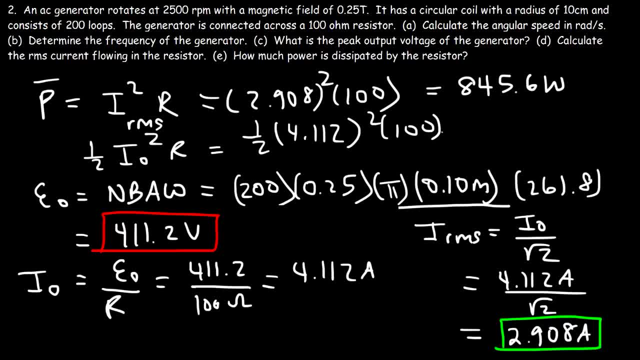 This should give us the same answer, And it does. Now, due to rounding, it might be slightly different, but it's 845.4 based on the way it's written. So this is the answer. So you could say it's approximately 850 watts if you round it to two significant figures. 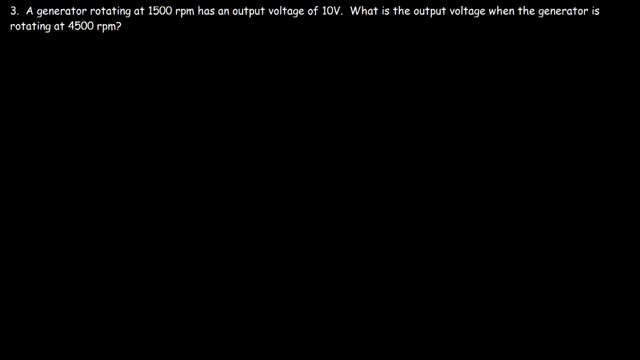 A generator rotating at 1500 RPMs has an output voltage of 10 volts. What is the output voltage when the generator is rotating? It's at 4500 RPMs. So here's the formula: The output voltage is equal to NbA times omega.